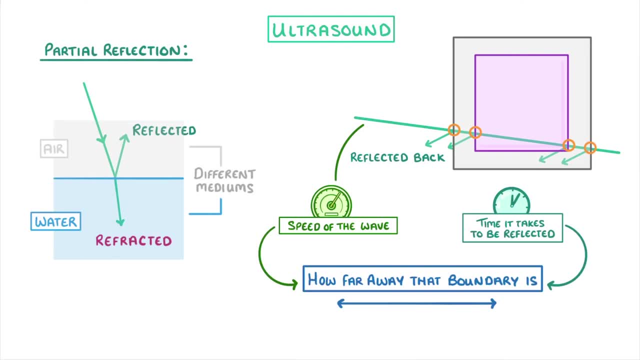 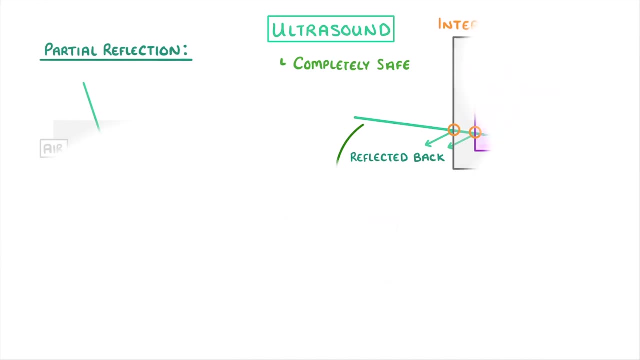 at the different boundaries within the object, which tells us about its internal structure, And, luckily for us, ultrasound is completely safe, so there's no need to worry about radiation or anything. The best known example of using this technique is probably in the ultrasound machines that 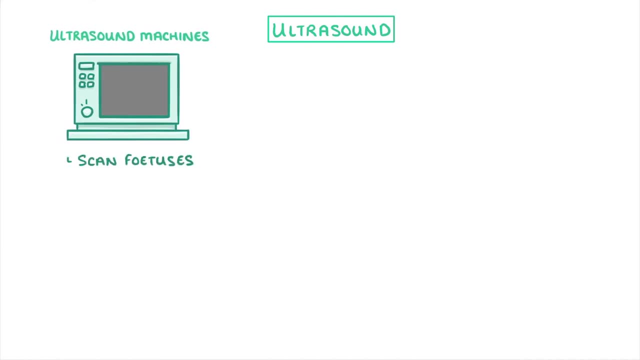 were used to scan foetuses. This works by placing an ultrasound device which can transmit and receive the ultrasound waves onto a pregnant woman's belly and firing ultrasound waves towards the foetus Every time the waves pass from one medium to another, like here, between tissue and 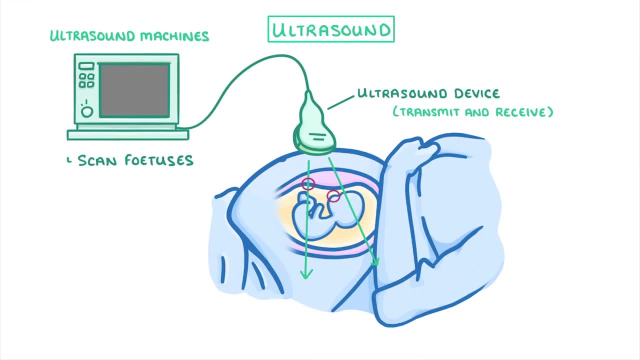 the fluid that surrounds the foetus, or here, between the fluid and the foetus itself. some of the waves are reflected back to the device And the timings and distributions of these echoes are then processed by a computer to produce a live image of the foetus, which can be used to check, if it's healthy. 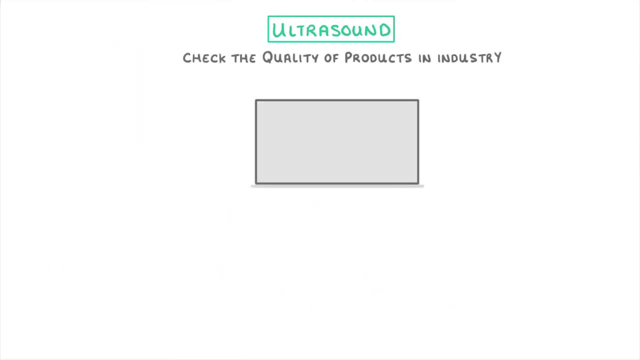 Another use of ultrasound is to check the quality of products in industry. If you imagine firing ultrasound waves at this object here, which should be completely solid, Well, if an object was not arms-sized enough to fit anywhere, then the supervisors would have to put bumpers. 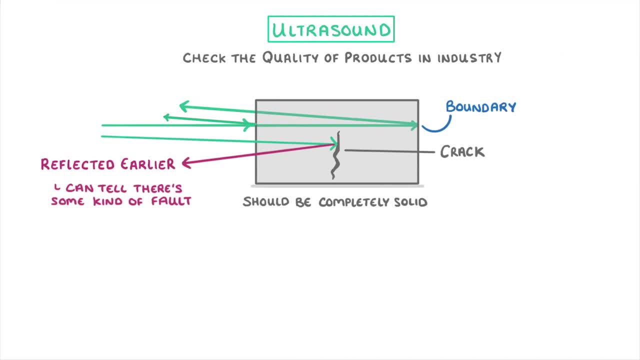 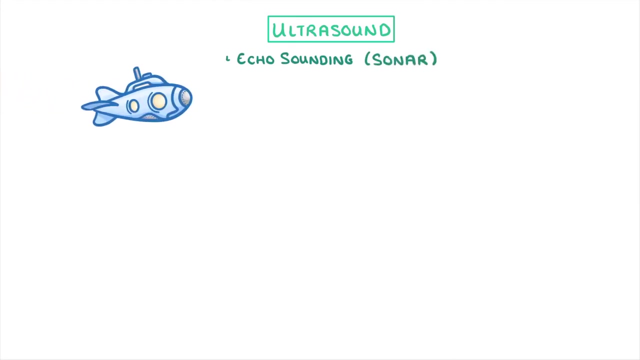 as a manual of all kinds, Not necessarily the same. with a single weakness It's worse than nothing. use we need to cover today is echo, sounding or sonar. This is where boats and submarines 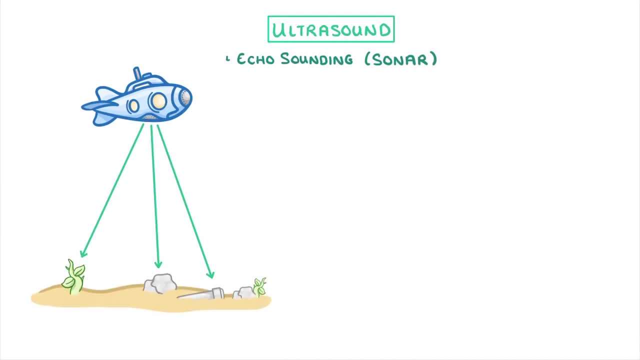 fire ultrasounds at the sea floor or other objects in the ocean to find out how far away they are. For example, if this submarine here fired a pulsive ultrasound that travelled at 1400 metres per second towards the sea floor, and it then detected the reflected,